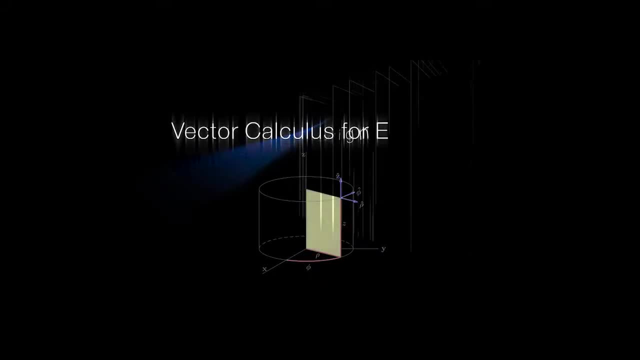 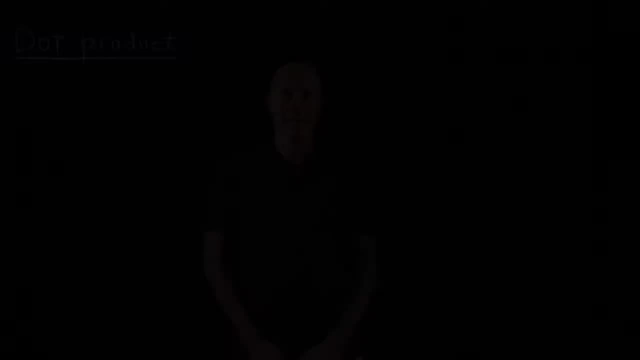 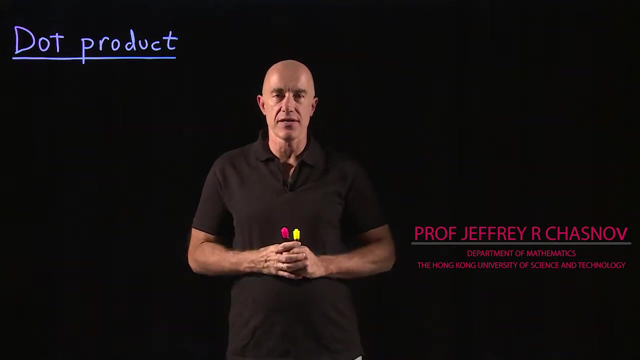 So we've talked about adding vectors. Now we have to need to discuss how do you multiply vectors. There are two types of ways of multiplying vectors. The first one I want to talk about is called the dot product. Sometimes it's called the scalar product, and that's because 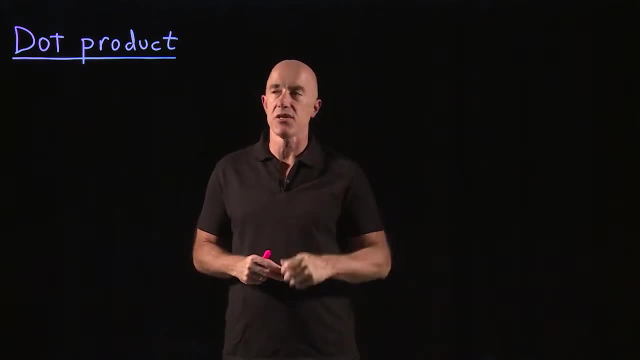 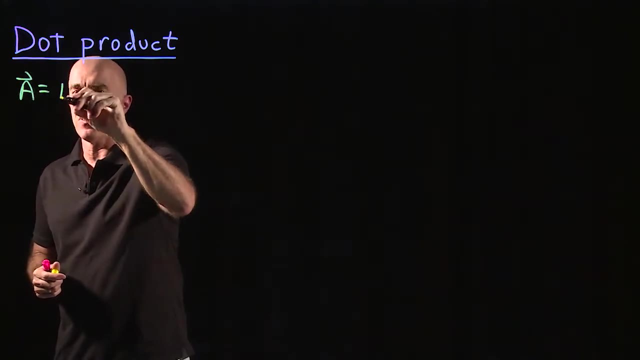 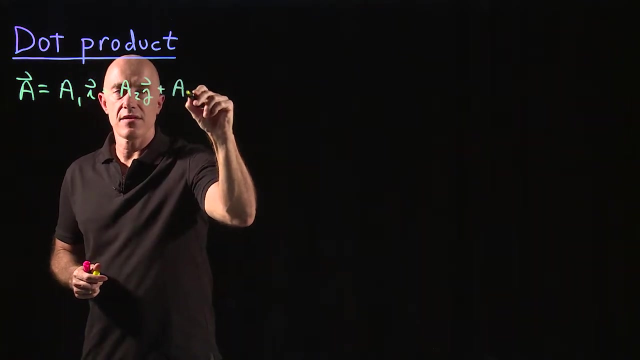 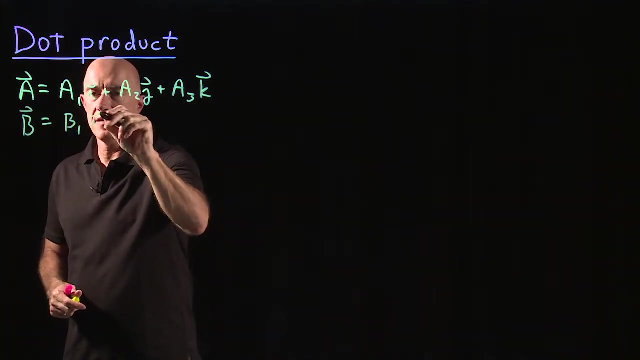 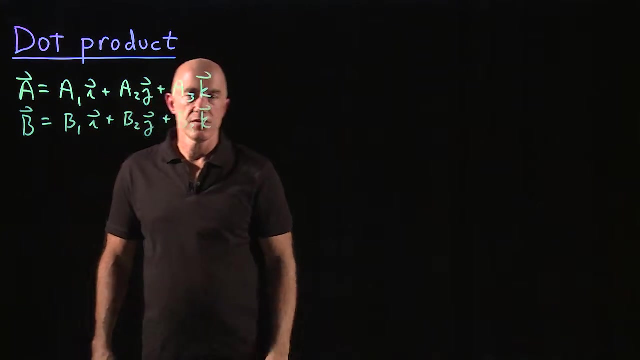 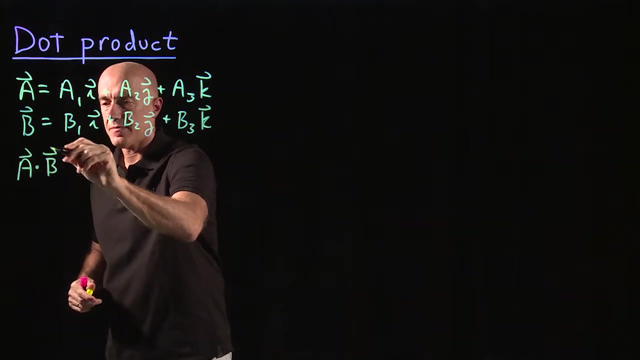 the multiplication of two vectors results in a scalar. So let's look at the vectors. Say A, we're going to write in component form as A1i plus A2j plus A3k, and B the same form as B1i plus B2j plus B3k. So the dot product then is written as A dot B is a scalar product. 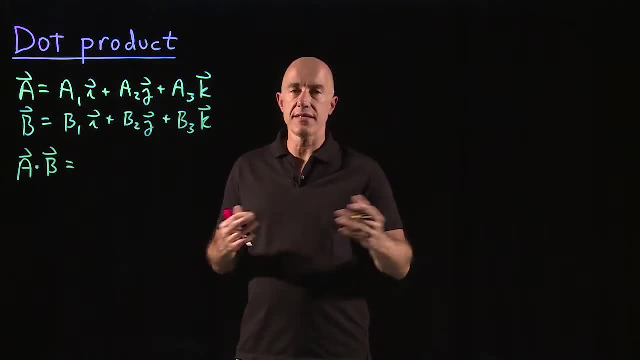 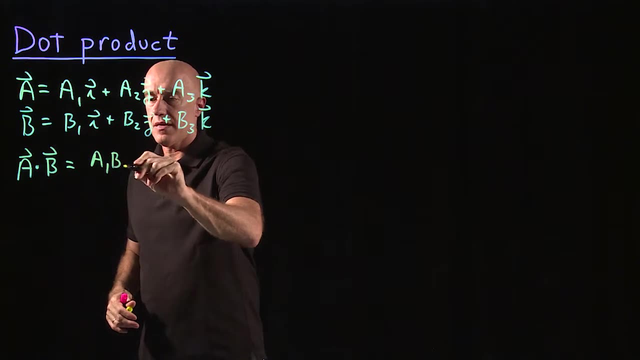 so the result is a scalar and quite simple. You multiply the components A1, B1, and B2. And A2, B2, and A3, B3, and then add them, So A1, B1 plus A2, B2 plus A3, B3. And that's. 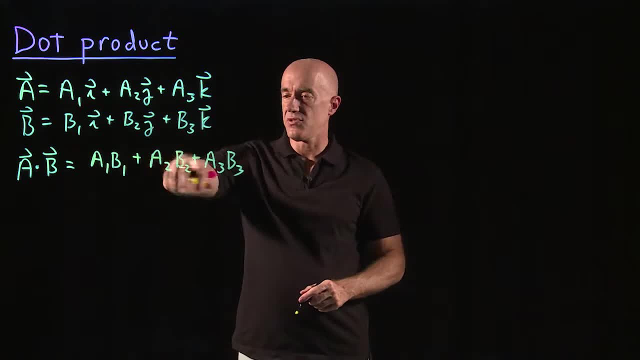 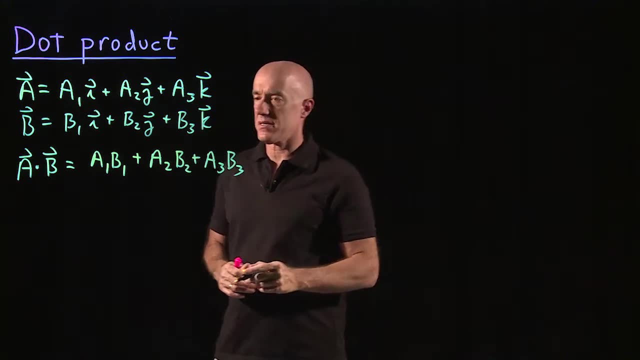 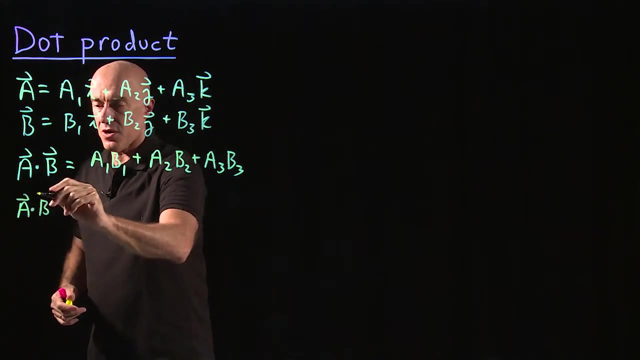 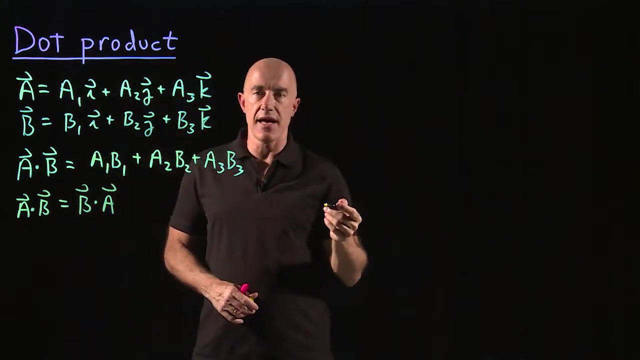 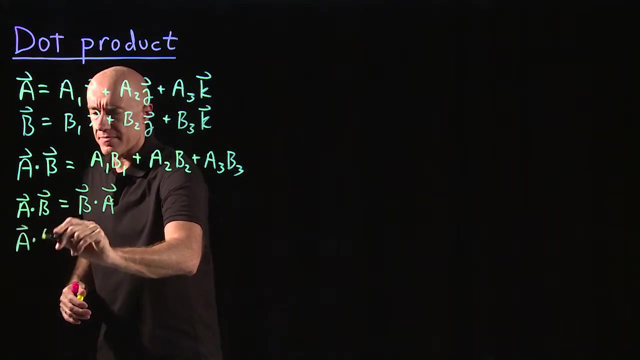 a scalar now, because there's no vector here on the right hand side. So what is the algebra of this dot product? It's easy to see that multiplication commutes. So A dot B is a scalar, A dot C is a singular vector And of course you can do that with a cube on. 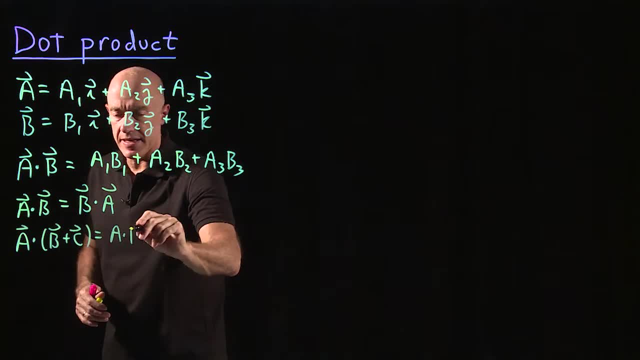 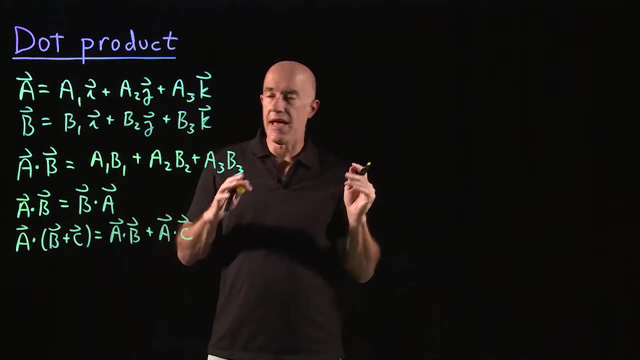 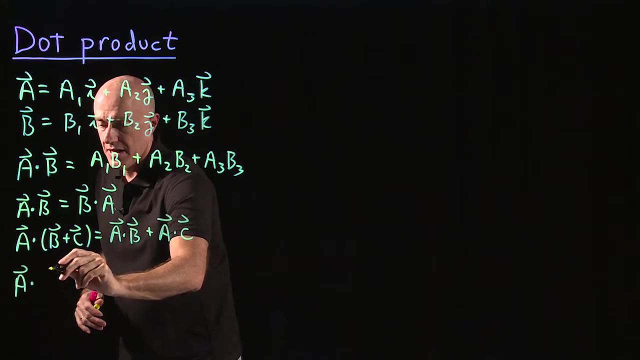 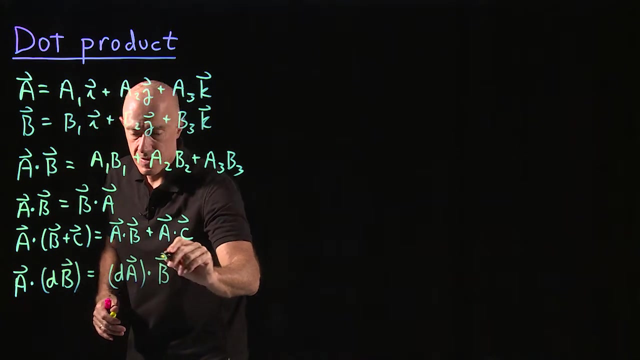 G across. So it really, really's like this. It's simple, right, Right, And that's you know. couple fingers for these. So let's do it one last time here. see that aa constant, let me call the constant d, say ad times b equals, d times ab is equal. 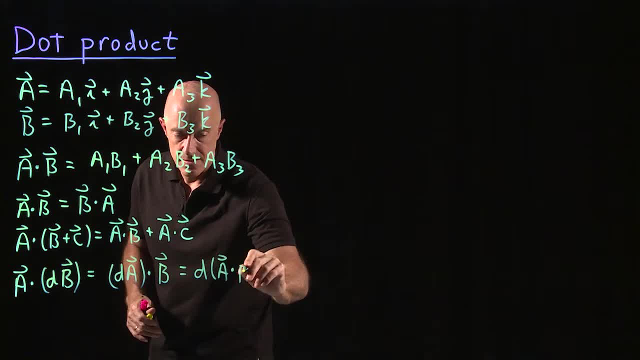 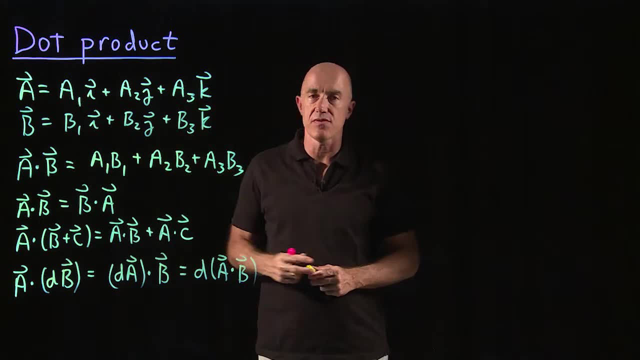 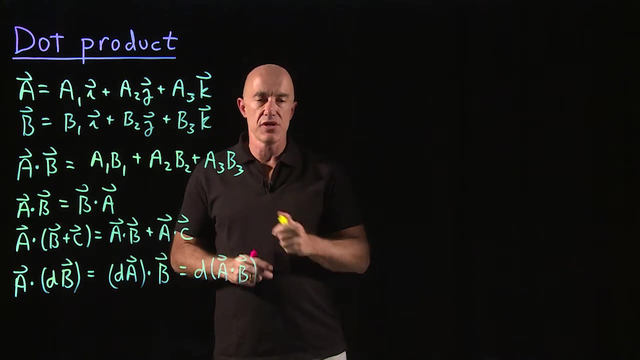 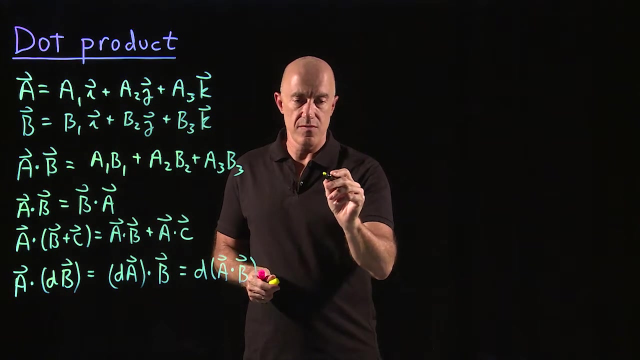 to d times ab. So that's the definition of the dot product and we see it's algebra. There's another way of defining the dot product that's a little bit more geometrically. So if we look at two vectors, so here's one vector and here's a second vector. 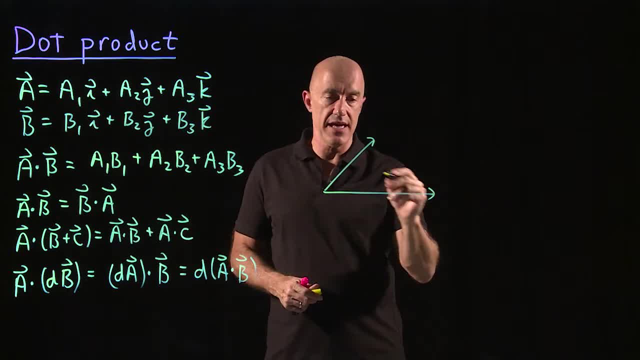 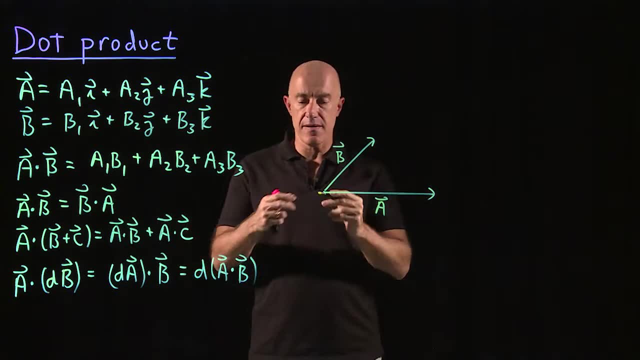 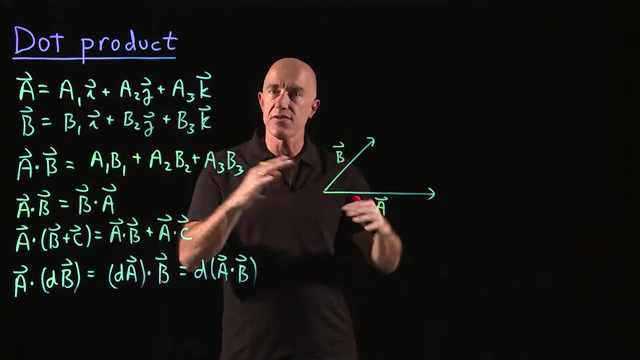 Okay, So let's say this vector is a and this vector is b. We can define a coordinate system to compute the dot product. So you're given vectors and you're free to choose any coordinate system you want. So let's choose the coordinate system that is where the x-axis is just the longest. 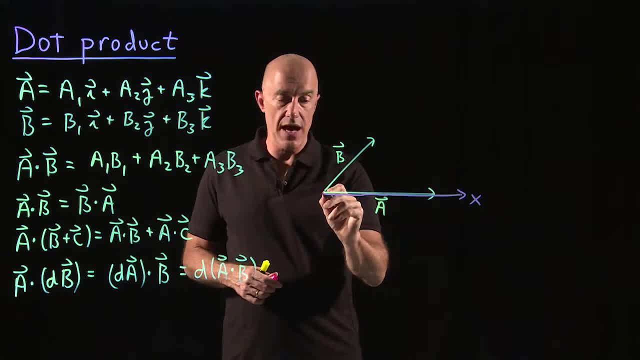 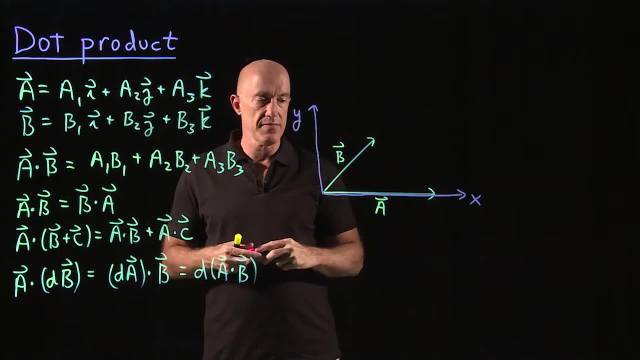 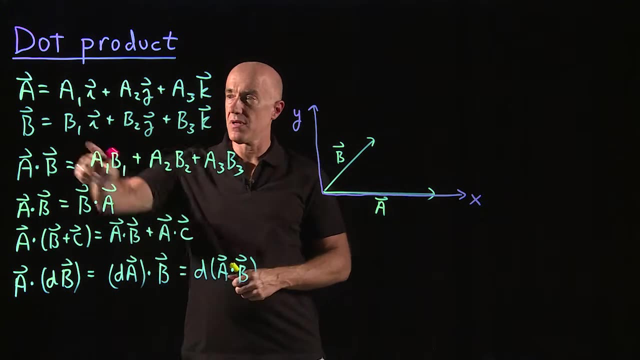 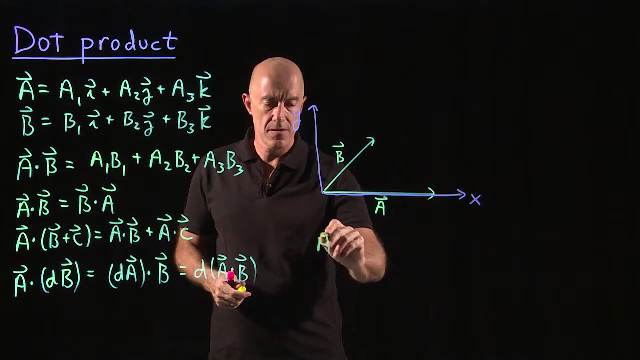 Along the a vector And then the y-axis is perpendicular. okay, We choose this coordinate system and then we can try to compute ab. So we have these components. So what are the vectors in terms of the components? Well, a vector right is along the x-axis. 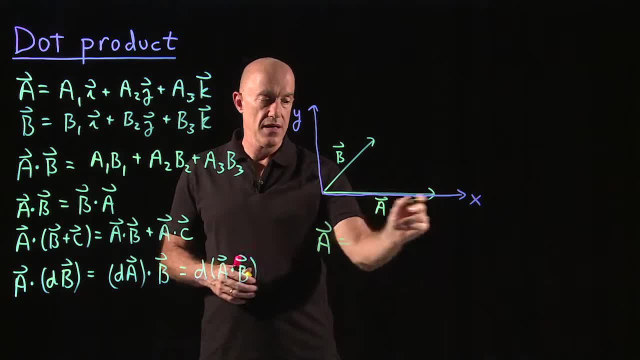 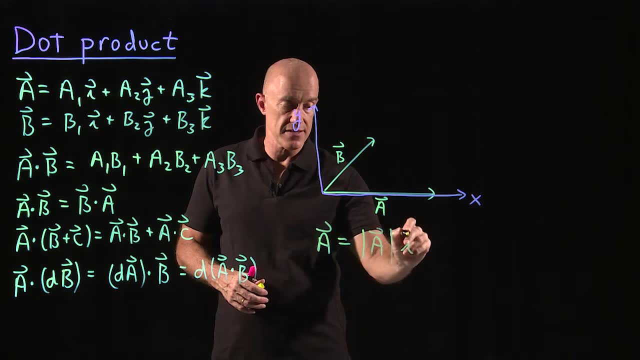 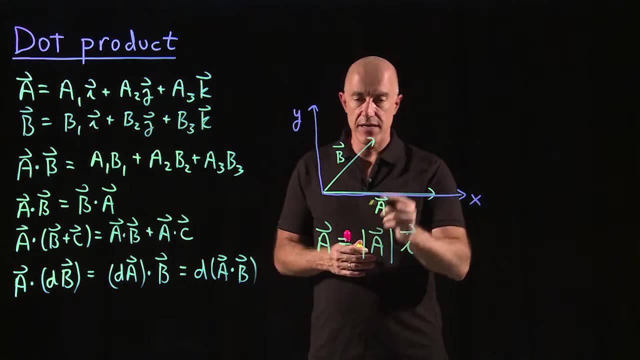 And it has a vector. It has a magnitude of a, So this is the length of a and it's along the x-axis. So we have the i vector. okay, What about b? right, So we can find the two components of b. 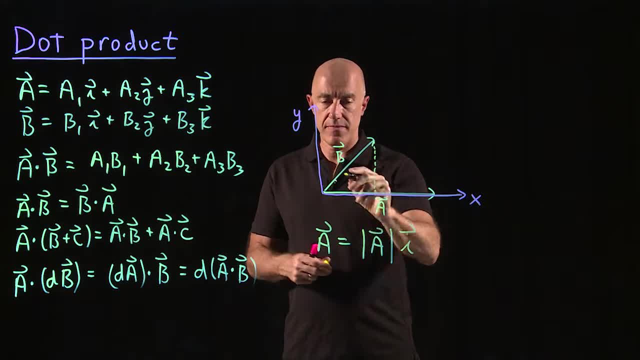 We can drop here, We can use some trigonometry here. So this is an angle theta. So the base here is the length of the hypotenuse times, the cosine of the angle, And the height here is the length of the hypotenuse times, the sine of the angle. 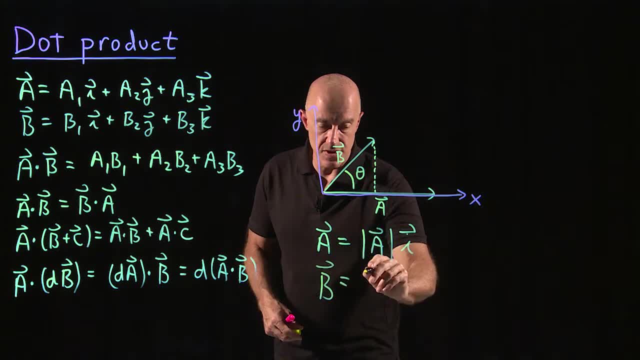 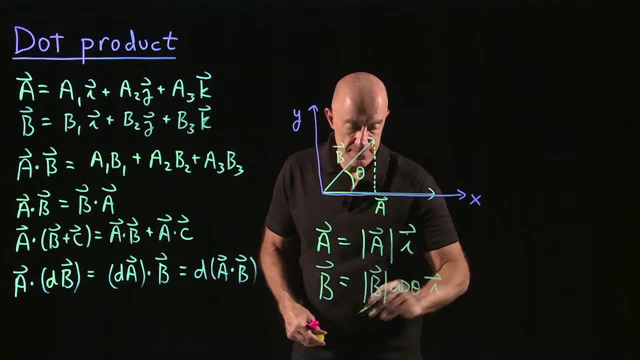 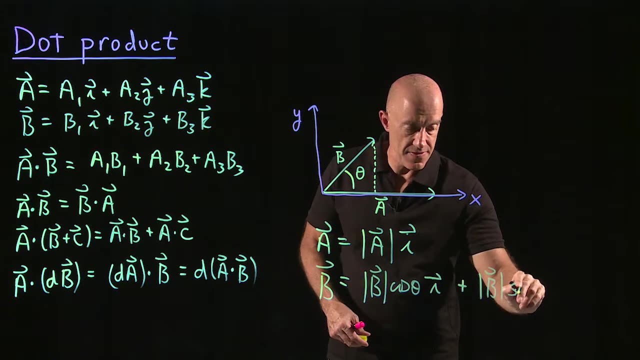 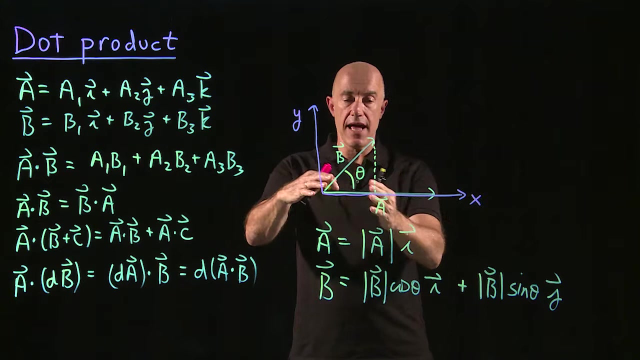 So b is equal to the length of b times cosine theta times i, Plus length of B times sine theta times j. okay, So by having two vectors, two arbitrary vectors, we can impose a coordinate system where x axis is along one of the vectors and the vectors lie in the xy plane. 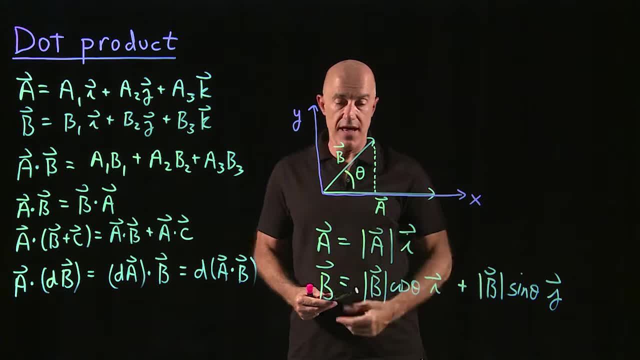 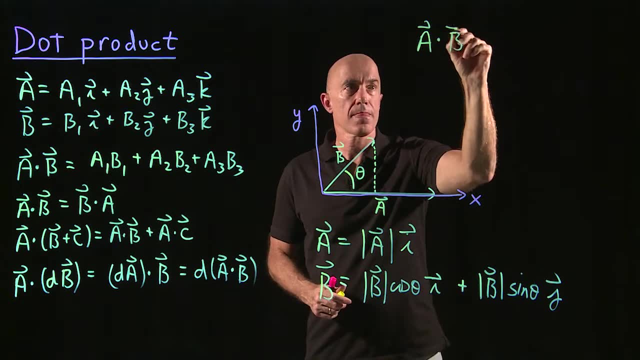 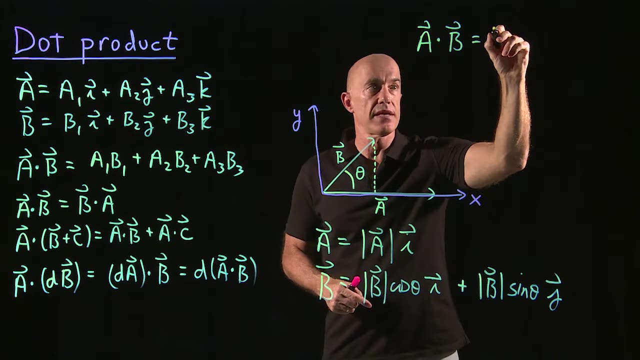 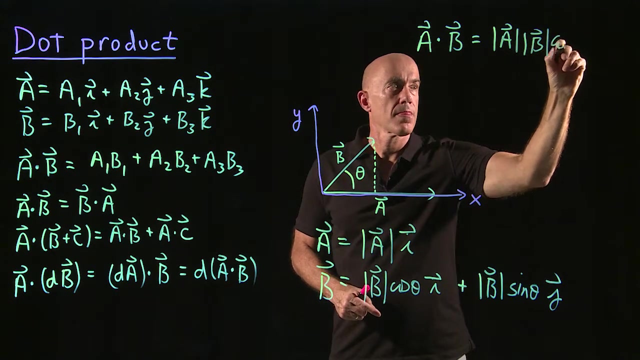 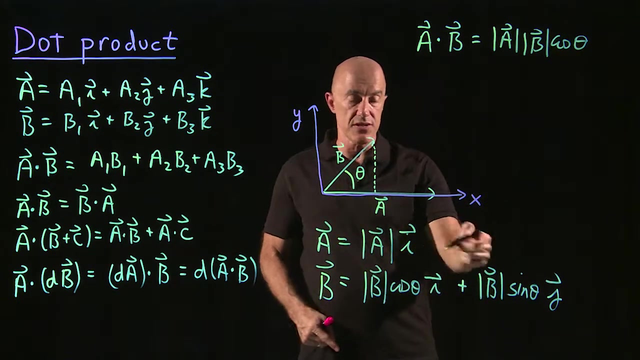 And we get this component forms of A and B And we can compute A dot B. So then A dot B is just the magnitude of A times the magnitude of B times cosine theta right, plus the zero times cosine theta. A dot B times B sine theta, because the j component here is zero. 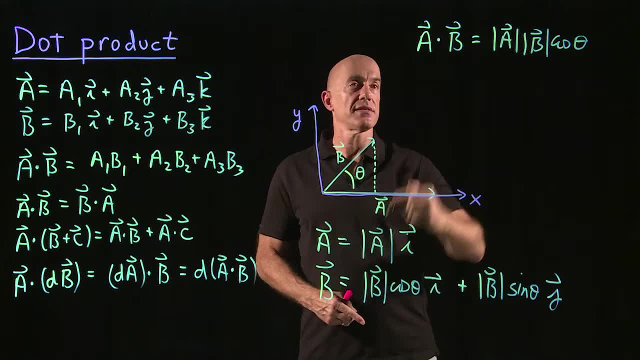 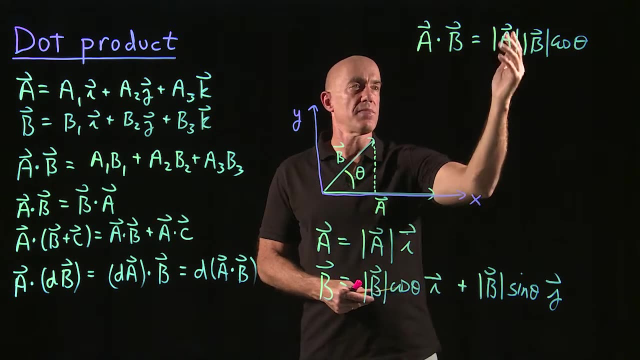 The y component is zero for A. So this is the dot product of A and B, And you see that this is independent of coordinate system. So this is true in any coordinate system. A dot B is equal to the magnitude of A times the magnitude of B, times the cosine of the. 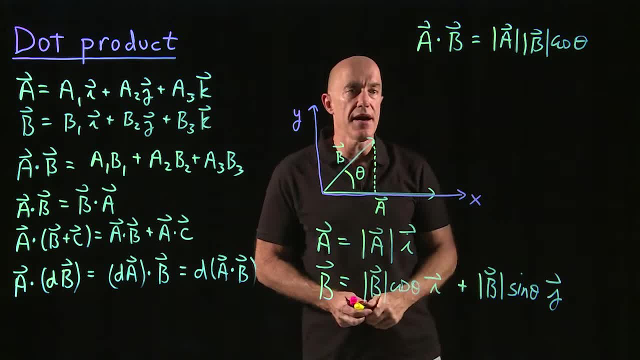 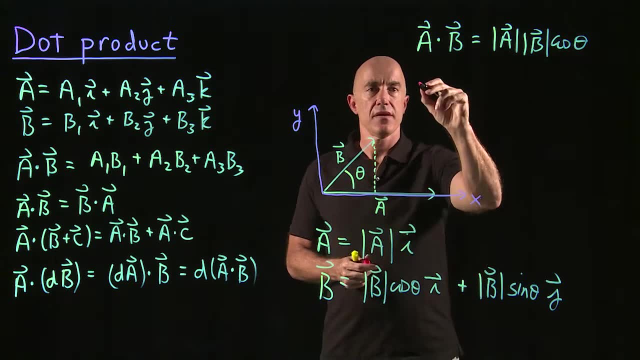 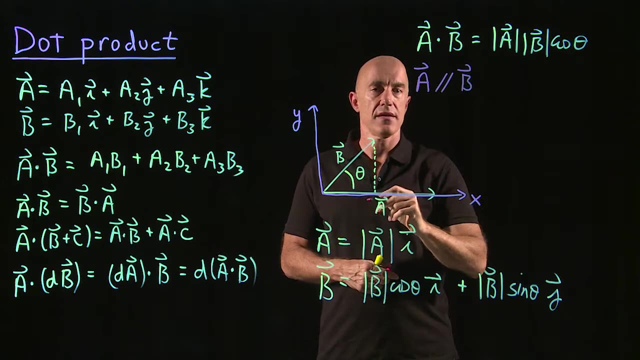 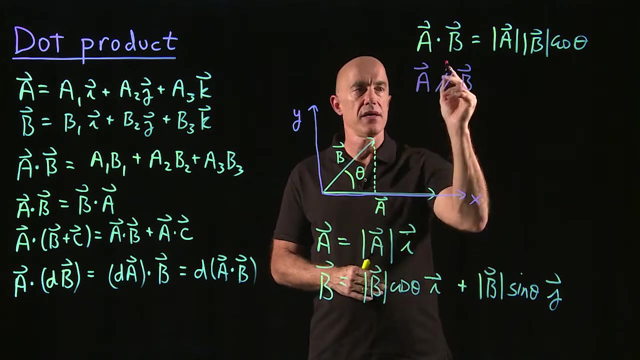 angle between them. Okay, There's two points I would like to make here. What happens if A and B are parallel? So if A is parallel to B, right, that means that B is a scalar constant times A. If A and B are parallel, B is a constant times A, Then A dot B is going to be. 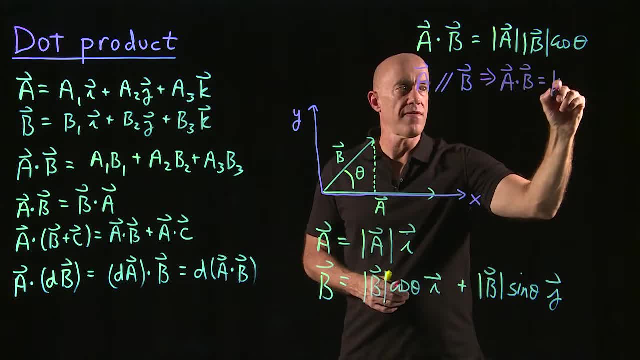 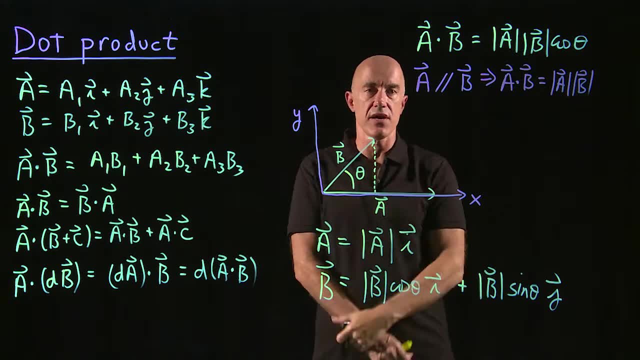 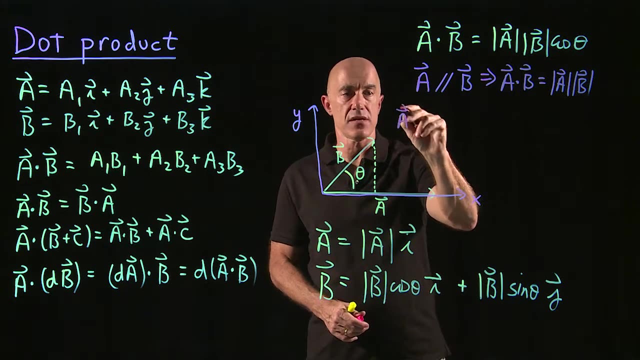 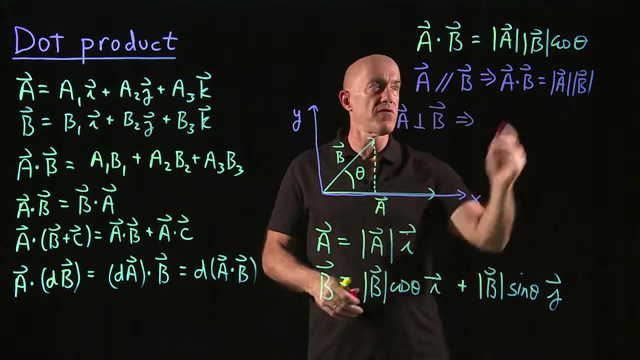 The magnitude of A times the magnitude of B. right The angle here is zero and cosine of zero is one. What if A is perpendicular to B? Then theta is pi over two and cosine of pi over two is zero. So that means for two.